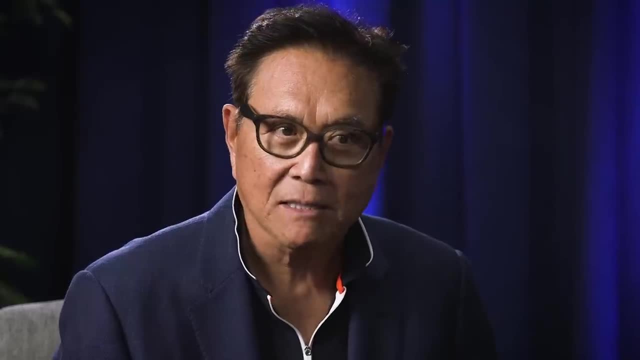 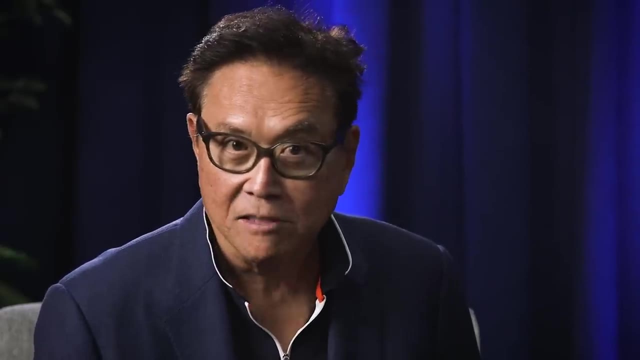 graduating from school don't even know what a financial statement is. And if they do, they probably had the same accounting teacher. I had, Mr Boring, who wasn't really an accountant. He had a master's in accountancy, but he had never been an accountant. So that's why I created the 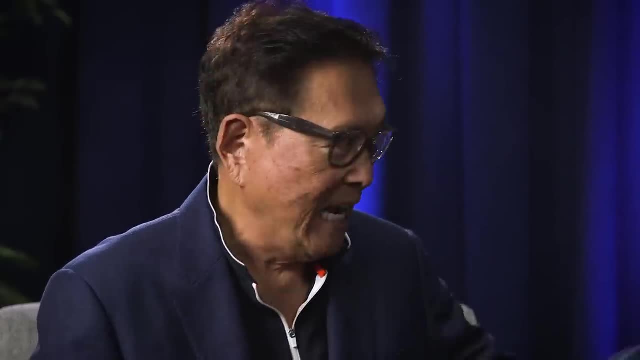 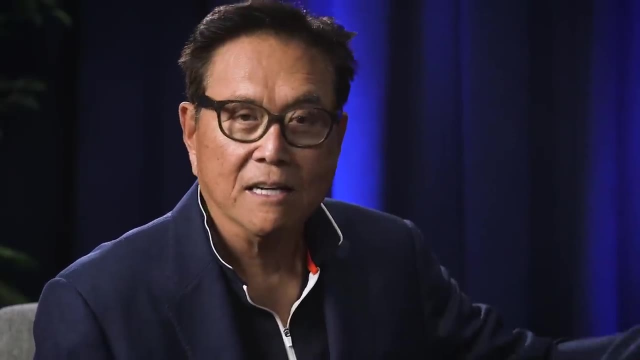 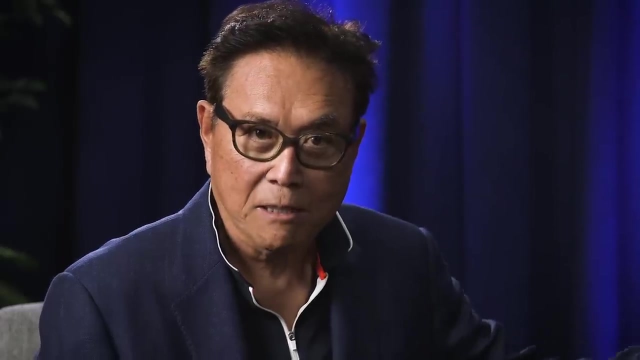 cash flow Board game, because accounting is the most important subject for individuals, because this is what your banker wants to see. Your banker wants to see your financial statement. This is your report card when you leave school. If you have good financial statement, bankers will give you. 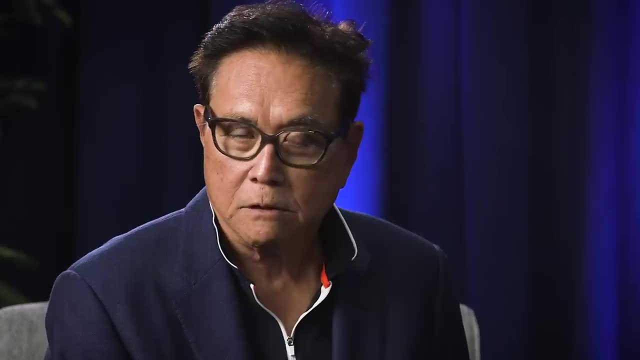 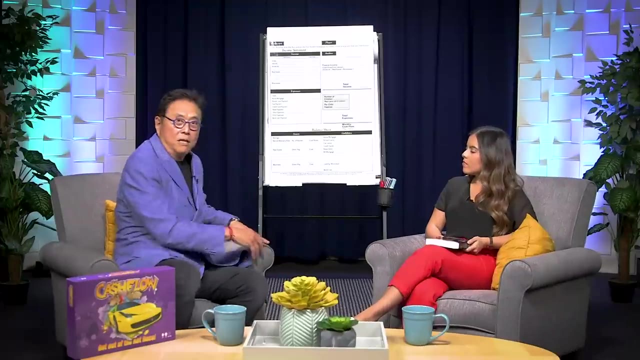 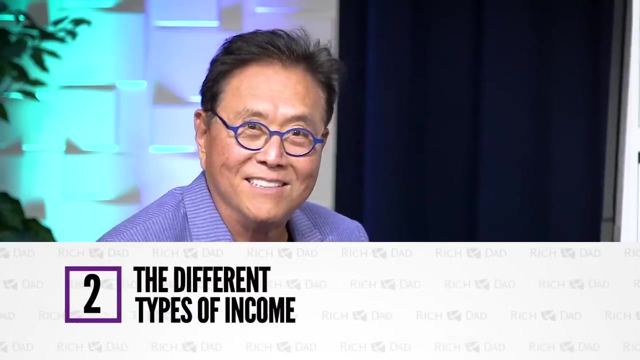 all the money you want. See, bankers have never asked me for my grades or my college I went through. I want to say this: You have this. they give you all the money you want. Point out really, really quickly The differences between what they're teaching in school and what we at Rich Dad teach. So this is the 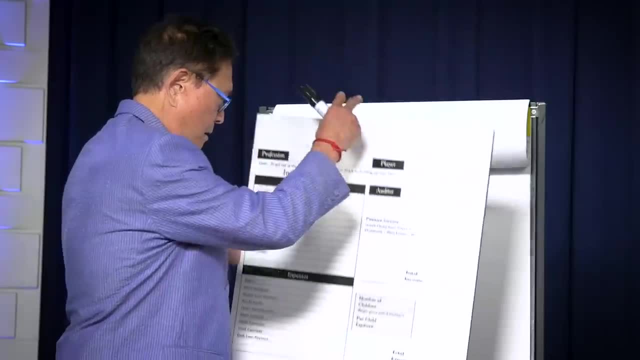 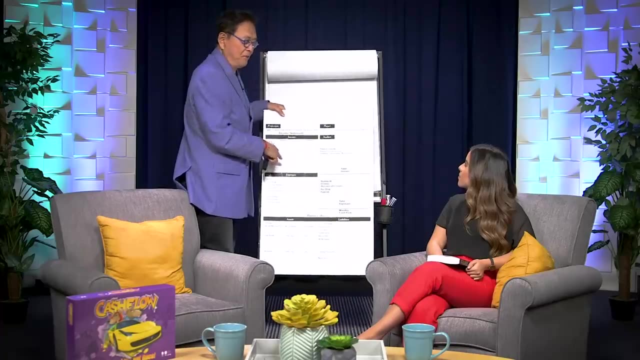 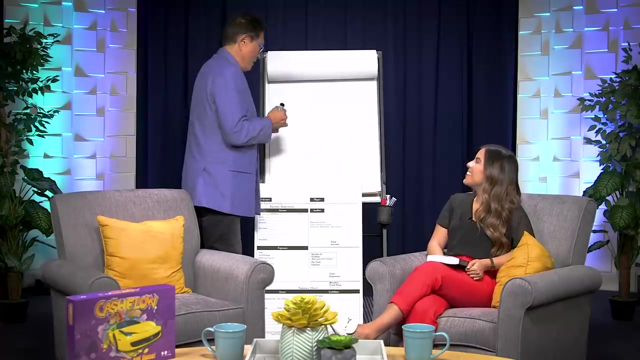 very big difference. Like I said, most school teachers are like my poor dad, And this was actually. this was Rich Dad, Poor Dad. What you're seeing here is a financial statement. You know, Rich Dad, Poor Dad is a book on accounting- the most boring subject on planet Earth, But book number. 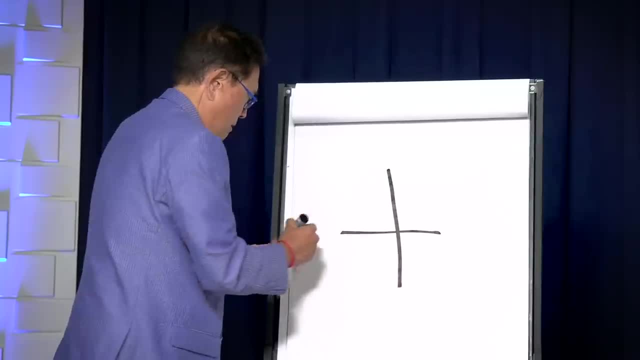 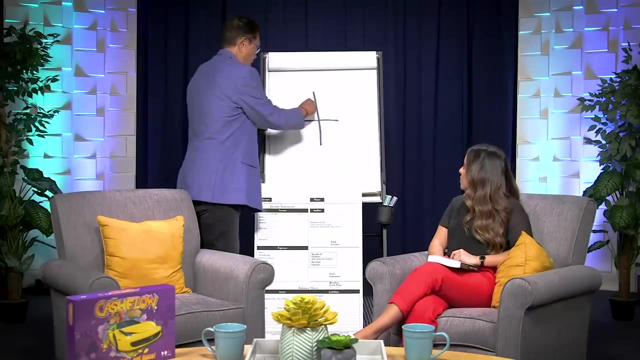 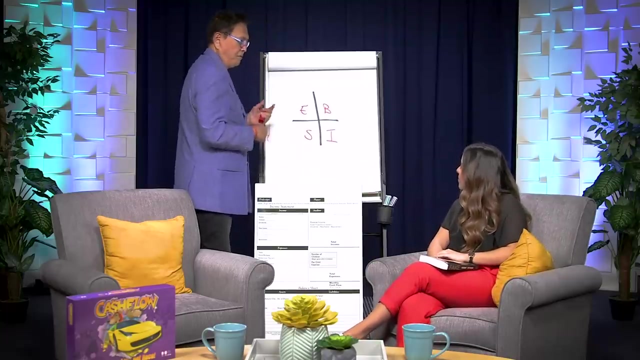 two of Rich Dad was this one here, And this was called the cash flow quadrant. right, You have E, S, B and I, So test for you. What does E stand for? Employee Good And what do employees always say? 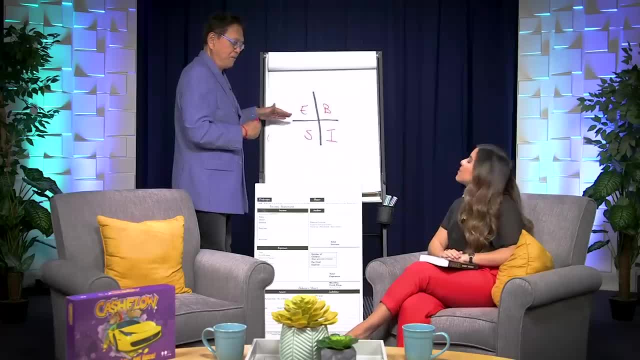 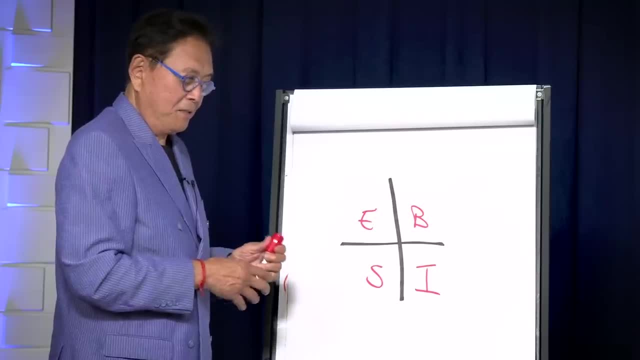 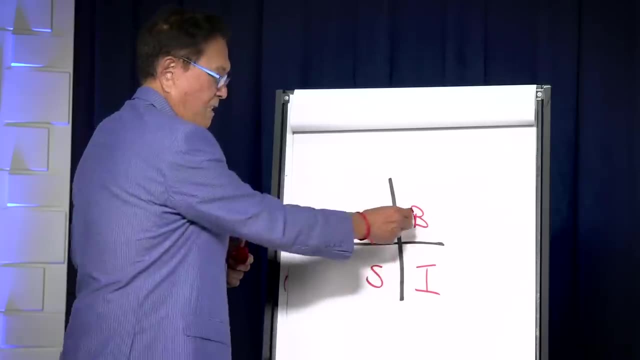 That they work for money, But they want job security, paycheck and pension. Yes, What does S stand for Self-employed? They're small business owners. Yes, Doctors, lawyers, They work for tips. They work for tips. So they're self-employed. And B stands for what? 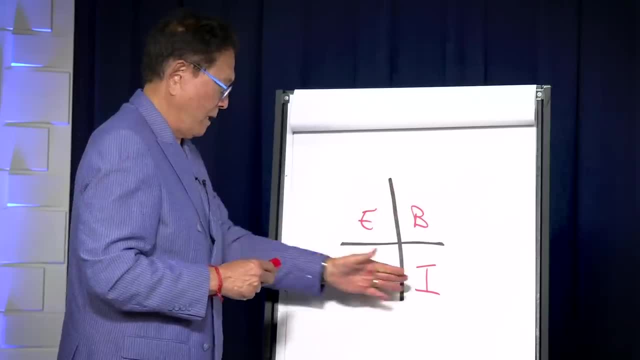 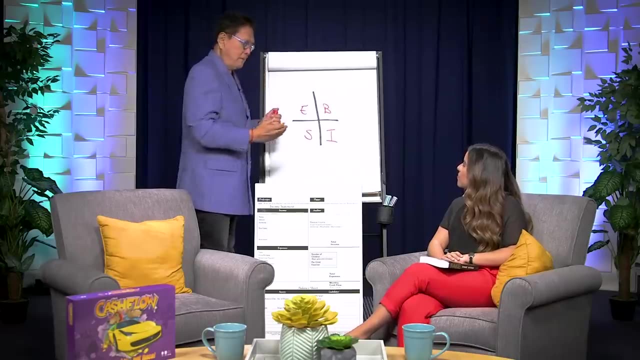 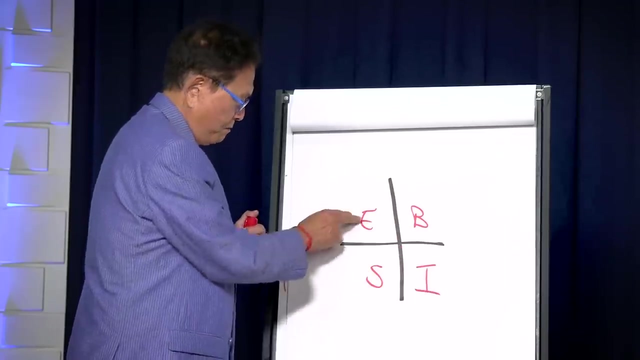 Big business owners, So 500 employees or more. And I stands for what Investor? Investor, It's more than just investor, It's insider. You see, this is like Shark Tank on the TV shows: These guys here have done this and they've done this. So this was my poor dad this side. This was Rich Dad here. 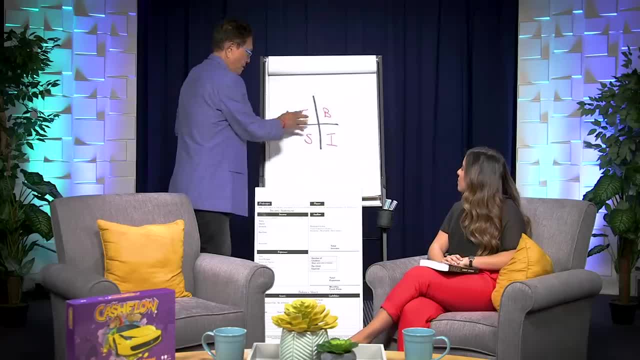 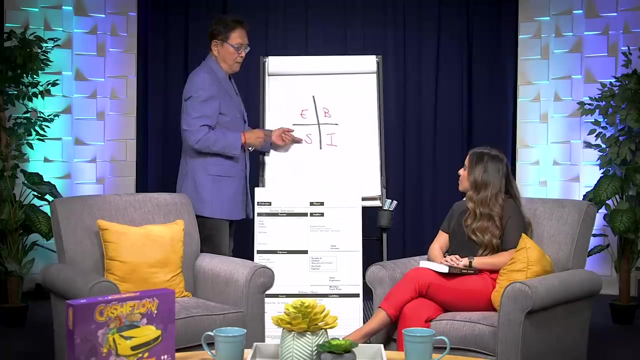 So the difference, that's what schools are not teaching, But what they're teaching you is. what's the difference between these people and these people? That's the big difference And that shows up. So when I was about your age, I had to make a decision. Did I want to? I was a pilot. Most of my friends wanted to fly for the airlines, But I'd be here Or I could be an Alaska flying fisherman around the place, A pilot with a small plane and flying around the world. 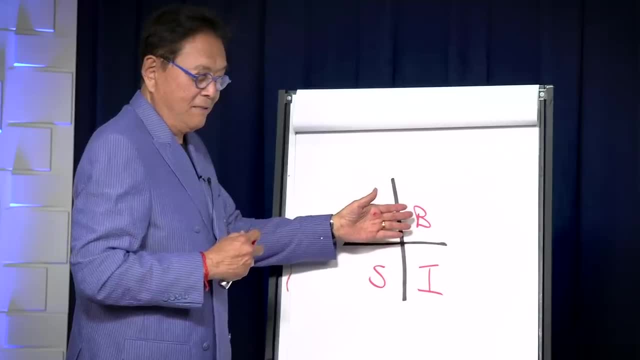 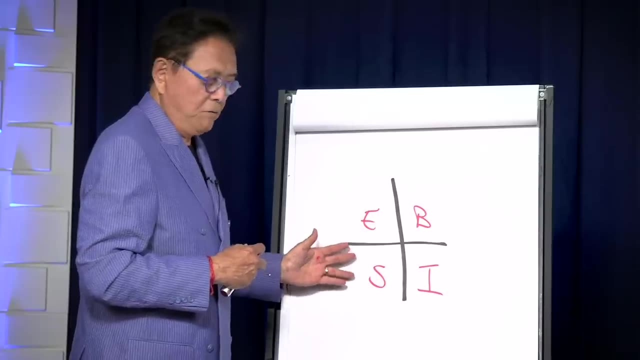 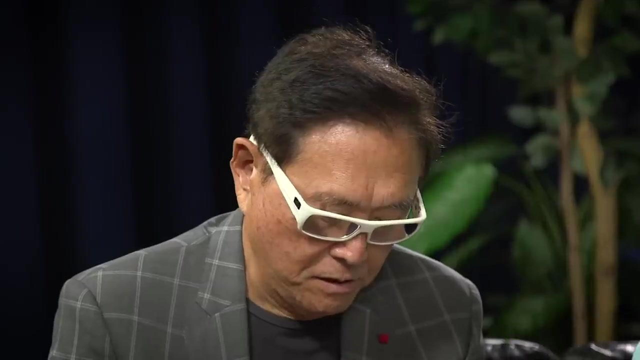 around the place, or I could own an airlines or I could invest in airlines, and that that's the difference in the mindsets and skill sets. you don't just make crossings. the education is extremely different on this side that on this side here- and I know most, most Millennials- they want a high-paying job. 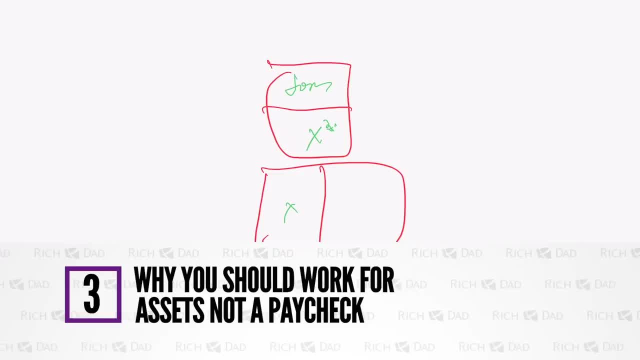 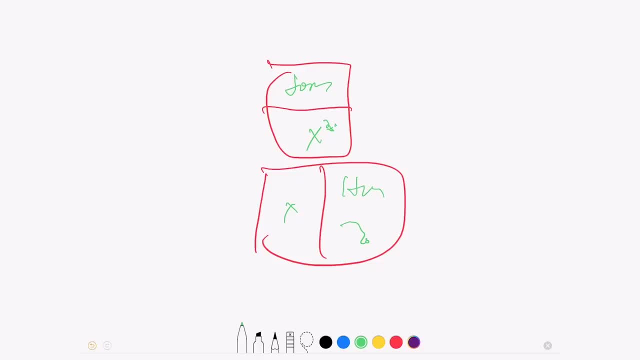 they want to be able to pay the rent, eat and all this stuff. and then you dream of the big house, a nice car and all that. but that's why 99% of Americans are broke, because their heads are on the wrong spot. so when I asked Kim if she 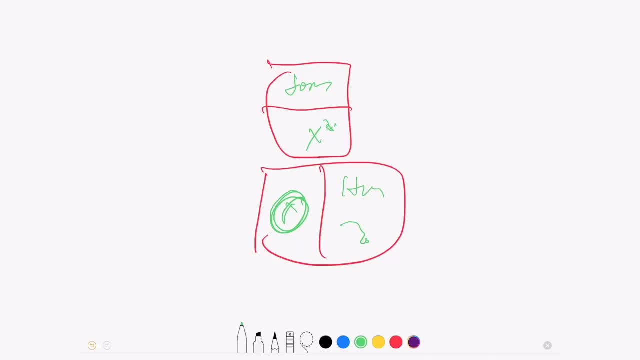 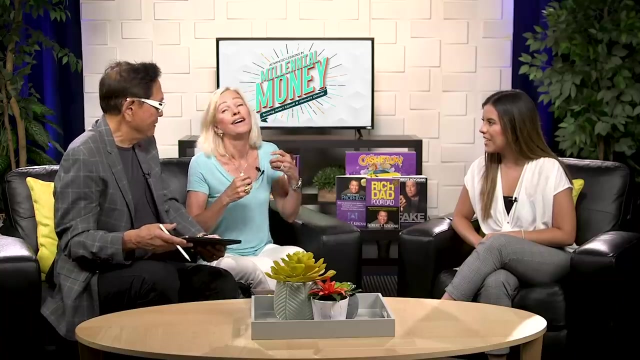 would take an accounting course was just two days. you know, I wanted to see if sure head could get into the asset column. that was a difference, wasn't it? yeah, actually it didn't happen right at that moment, but it it's, you fell in love with me. 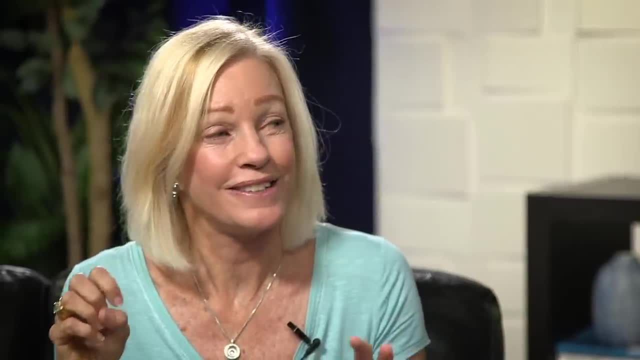 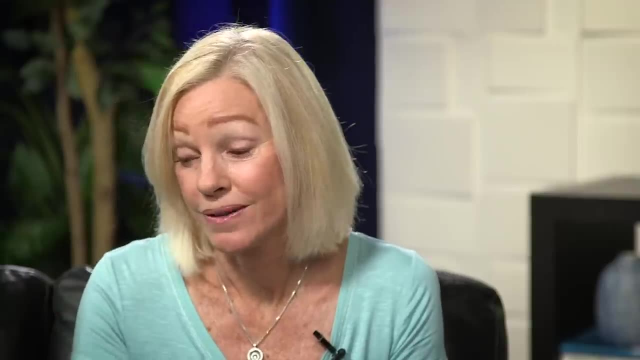 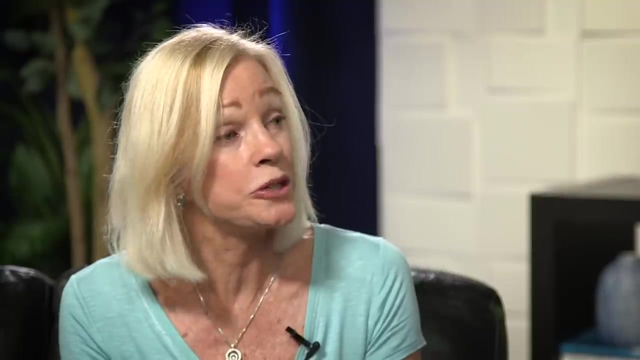 but this started. this started the journey on investing, the start of the journey on assets. but I do remember the moment down the road where, just like everybody else, I was focused on the income column: getting job, get the pay raises if you're an hourly rate wage, work more hours or raise your hourly. 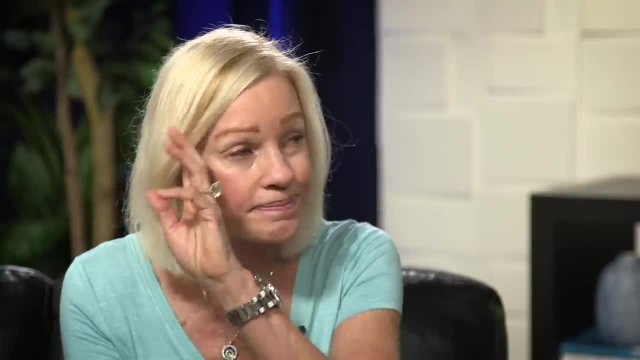 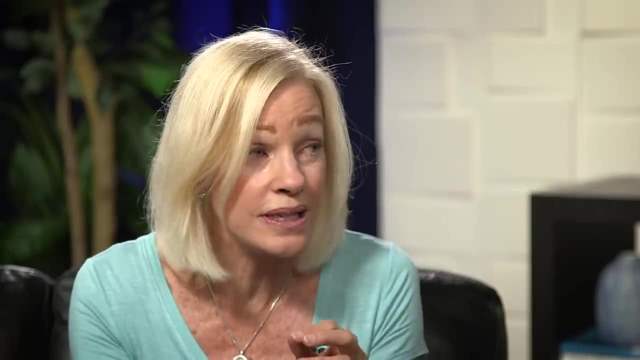 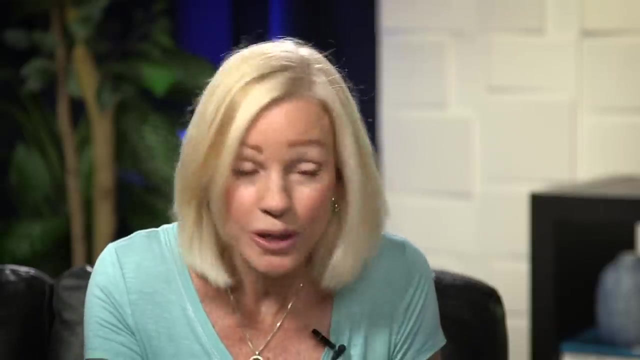 wage. so I was always focus here. and then, finally, after we'd actually bought some investment properties, the light finally went on and I'm like, instead of focusing on acquiring income, what if we focus on just acquiring assets, that the assets go into the income, like this? so that was a huge shift in my mindset and 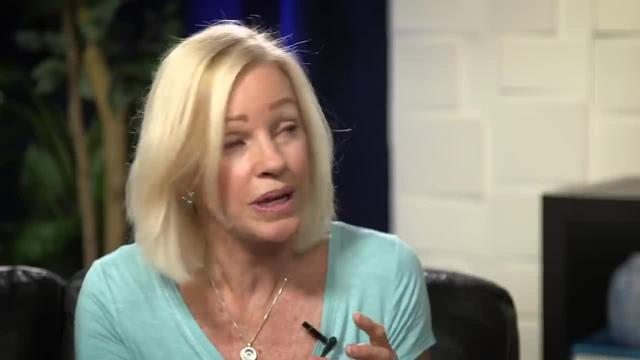 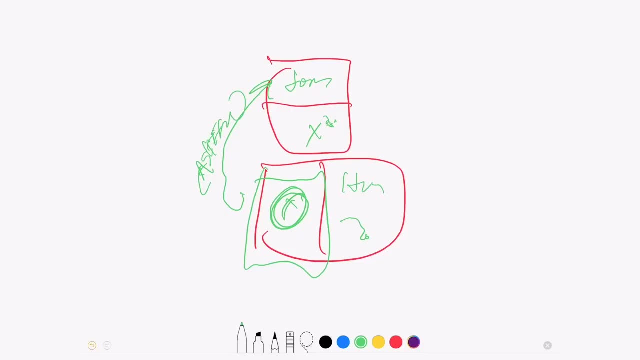 once that shift happened for me, I don't think about the income column anymore, I just think about the asset column and that's and that's our game called cash flow. yeah, and so when Kim and I met, we had nothing. it took us ten years to go. 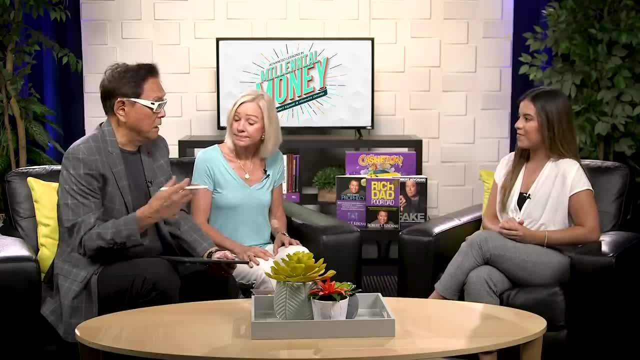 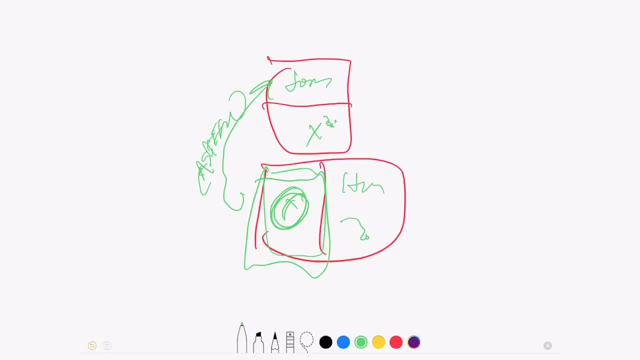 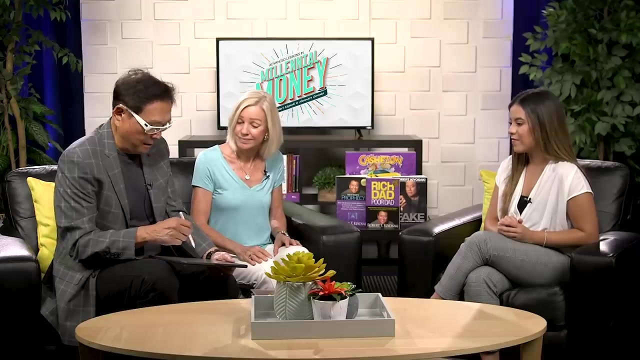 from nothing to financially free. so she was 37, I was 47. but that's the power of focusing on assets versus liability. most people are so busy working for money, so busy trying to pay their bills and so busy buying liabilities. I think our assets. so my first gift to Kim was the counting game to get her head in here. 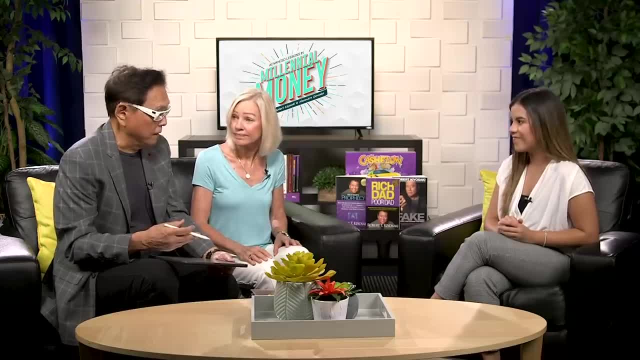 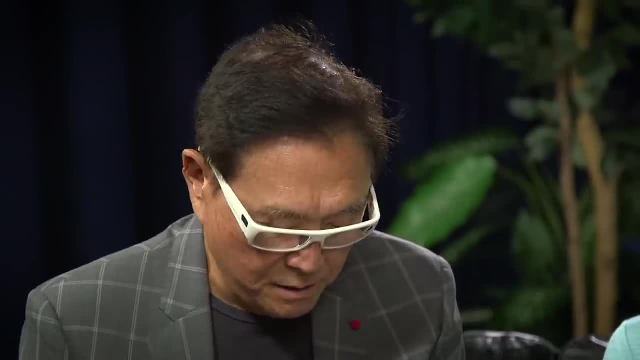 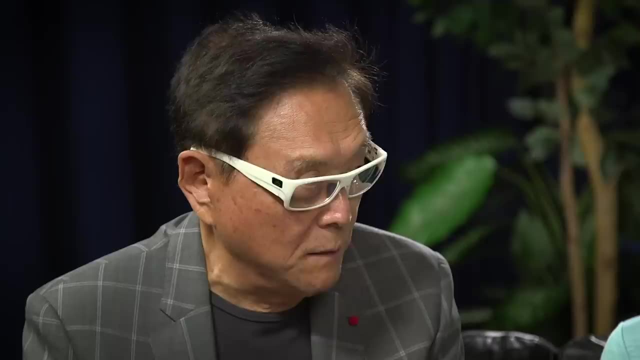 and today we're financially free and that's the whole thing. you so everybody can do it. it's a matter of putting your head into the right column. and then for me, it was in 73 I took my first real estate investment course. here I'm free. you know, I lost money, get made money back, but I never. I never got out. 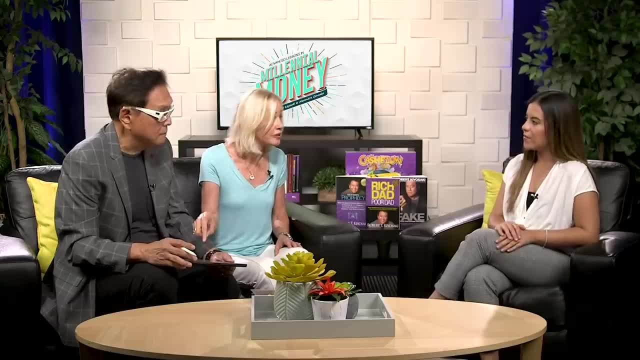 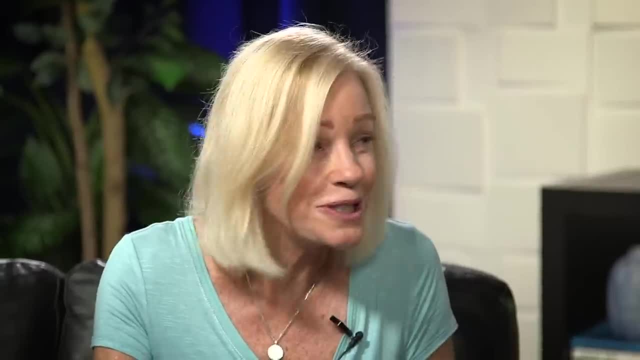 of the asset. we're still- I mean, we're still- practicing here every single day. I'm working on a new project right now in the asset column. it's gonna put a lot of cash flow into the income column because, again, we're focusing on asset, not the income column. there's three kinds of money today. you guys got to be 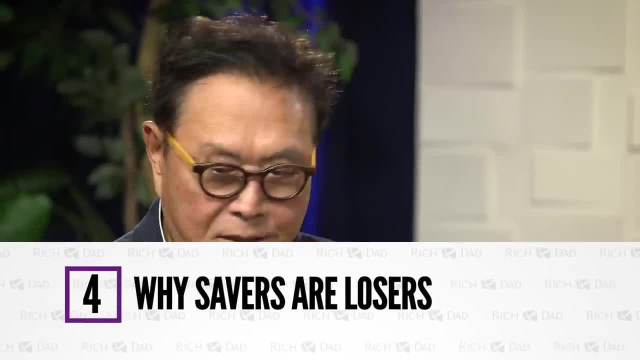 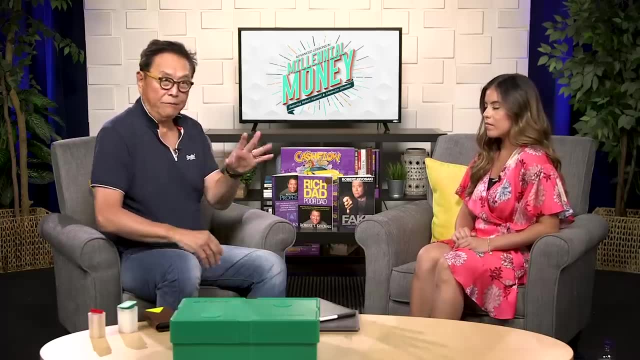 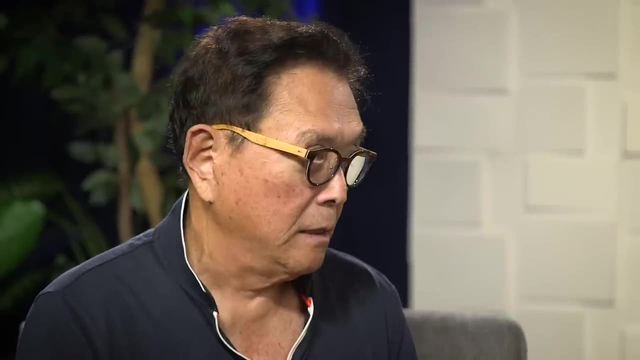 aware of one is God's money, and God's money is gold and silver. so this is silver and this is gold. the reason I brought is most people don't know what it looks like. and then there's government money, which is Fiat currency, which is the dollar, the yen, the peso, the euro, the yuan. yeah, fake and everybody's. 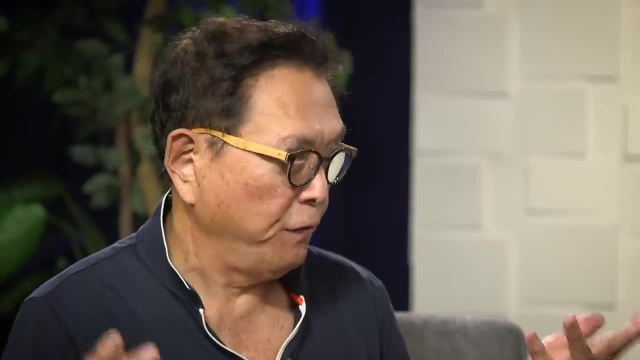 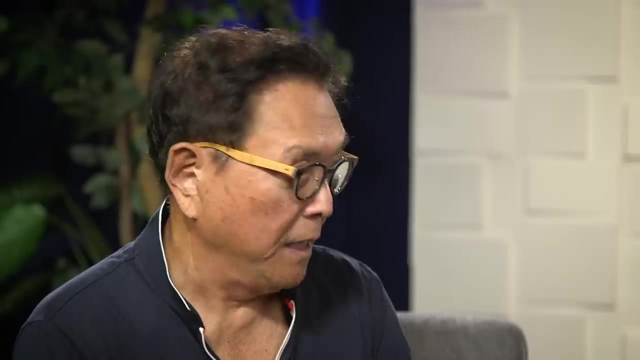 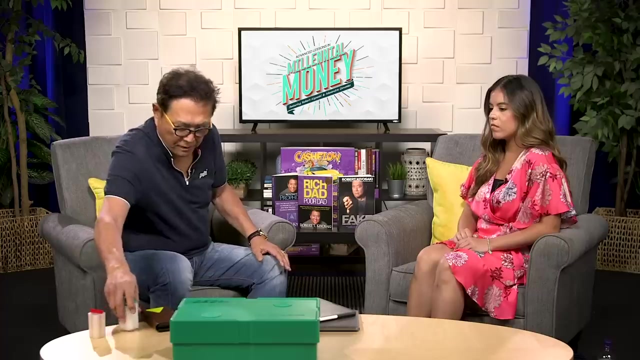 working hard for it. it's like eating fake food or drinking fake water. that's why people are getting sick financially, because they're working for fake money, okay, and then there's fake assets, which was another part of their fake millennial, the fake generation series. but the reason I brought this here is: 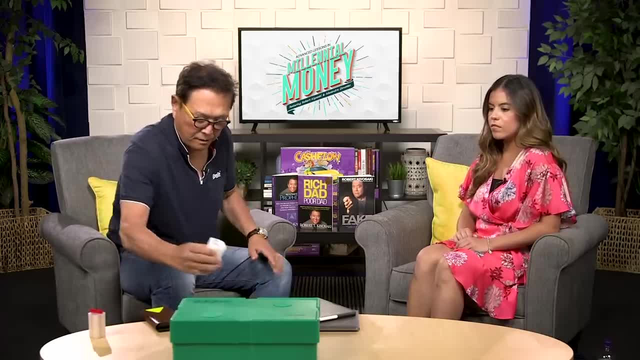 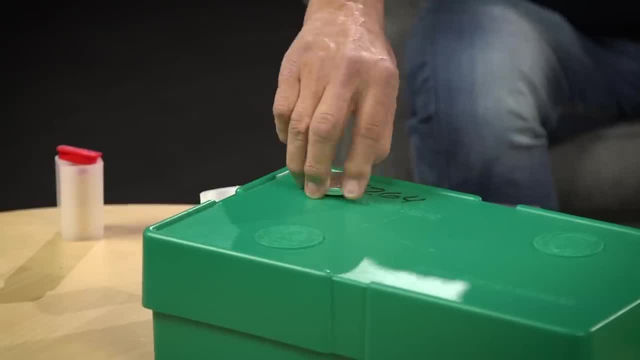 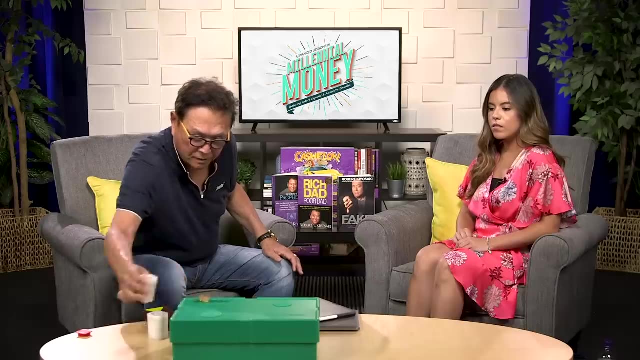 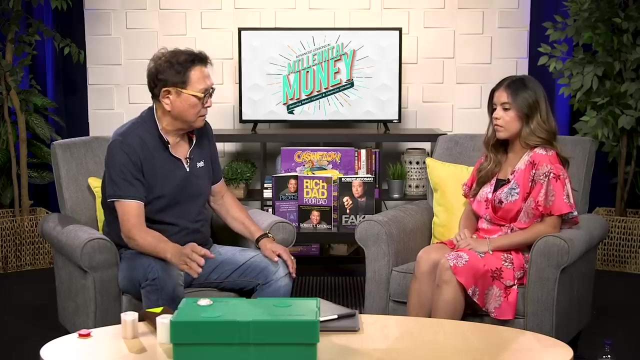 most people haven't seen it. this here is real silver plata. that's what it looks like. and so in 1972, and this here is gold. this is God's money. this is what God's money is looks like. the reason I call it God's money is: you can't fake it, you know you. 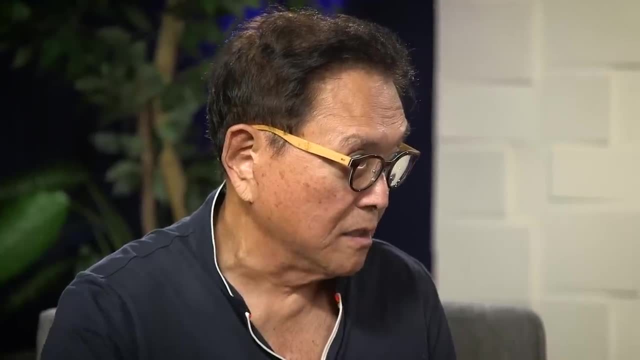 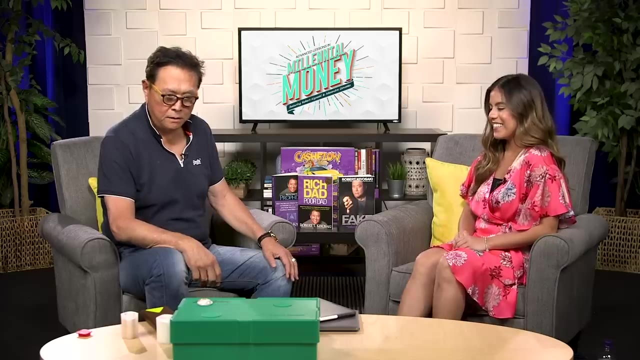 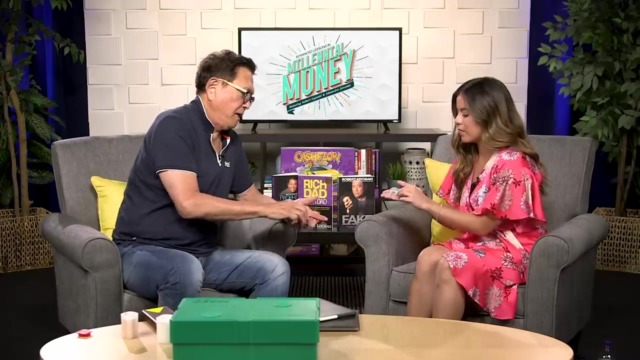 can fake it with a fake ETF, like a gold ETF or a silver, which I don't touch because it smells as bad as the guys that printed that crap. you know, I mean Jesus, but this is real money. so you look at this here. when I first started buying, 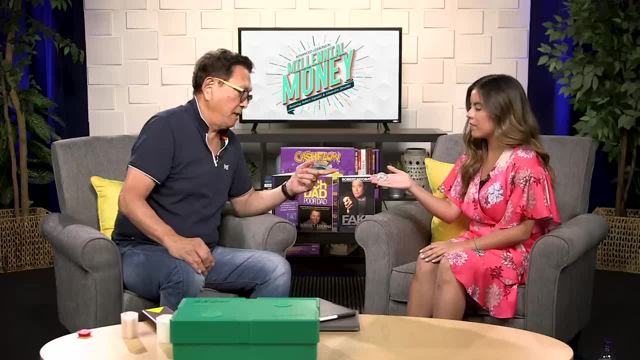 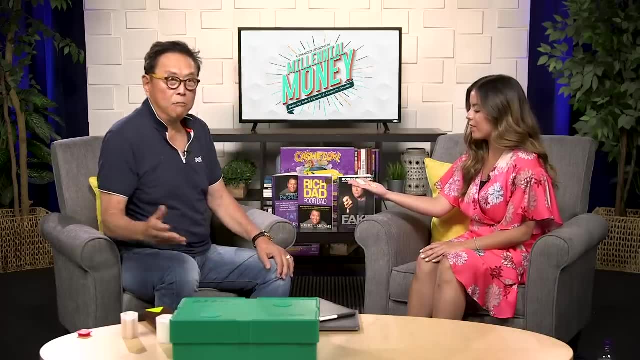 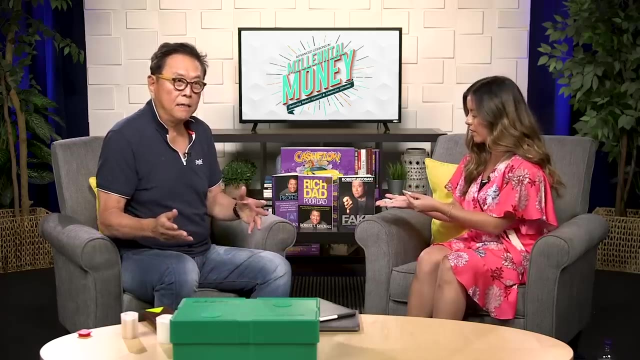 that that was a dollar forty. yeah, today that's sixteen dollars, and this here is auto gold, and the reason we brought it is most people haven't seen or touched. this is real. this is God's money. why did I say it's God's money? because he was here when the earth was created. yeah, and it'll be here when. 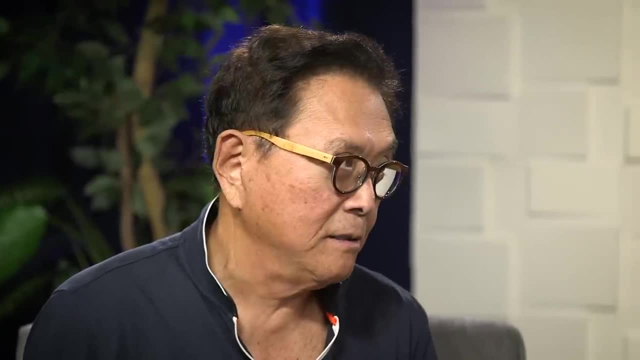 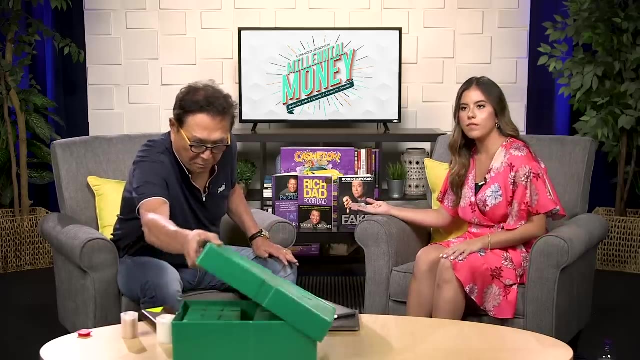 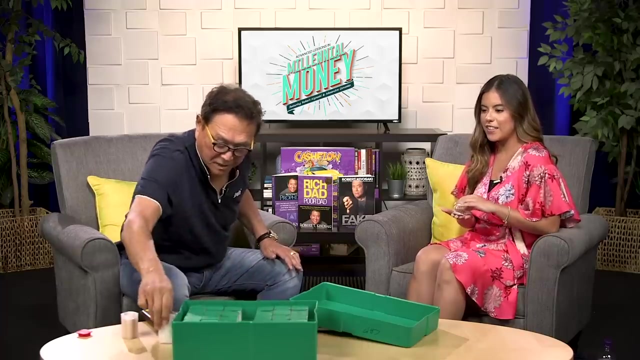 we're all dead and gone. when you're saving those fake dollars, this will still be here, yeah, or those fake ETFs or those fake stocks. so this here is called the green box. these are. there's 500 of these little tubes like this. Wow, 500 coins in here. 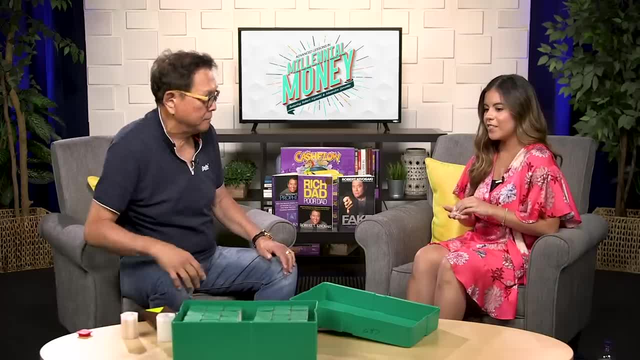 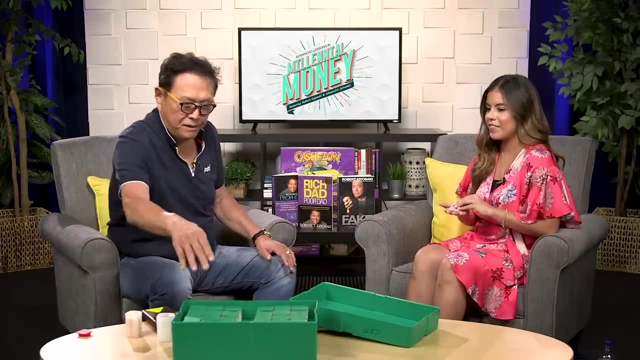 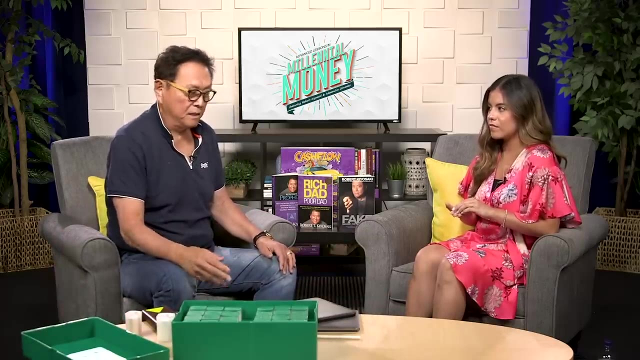 and this is one which is worth more. which ones are for more the gold? yeah, this is worth more than all that. now, the reason I say this is because, for your generation, this could be the biggest opportunity you'll ever see. I'm not making any commissions on this, yeah, but if you look at what happened, 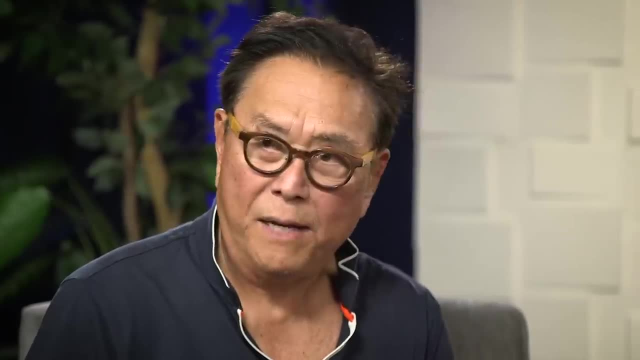 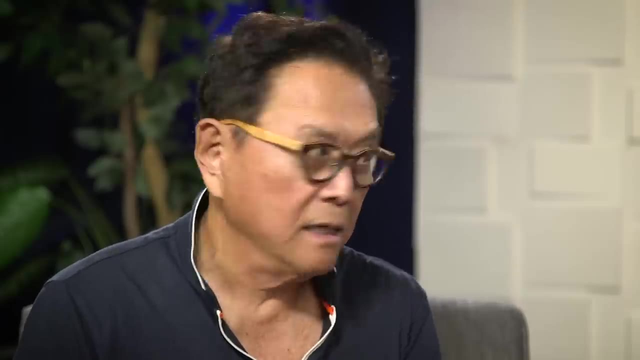 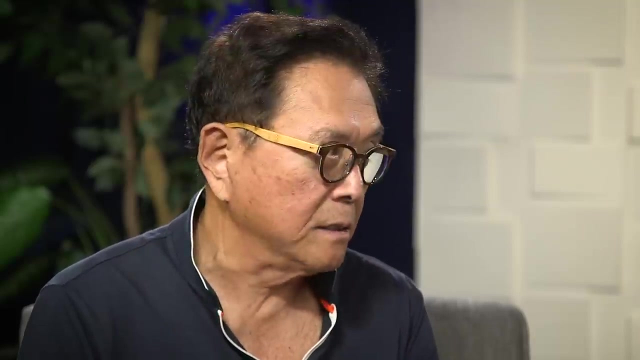 with the fake central bank. see the purpose of the central bank or the Fed or all you know, the the Japanese that the Bank of Japan or the European Central Bank. they pump out fake money. the purpose of central banks like the Fed is to protect the banks, not you. they're a criminal operation, as far as I'm. 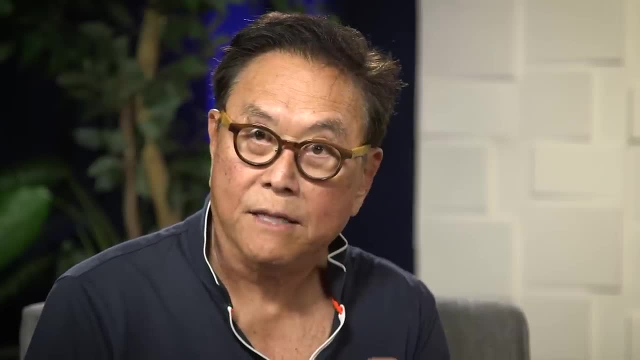 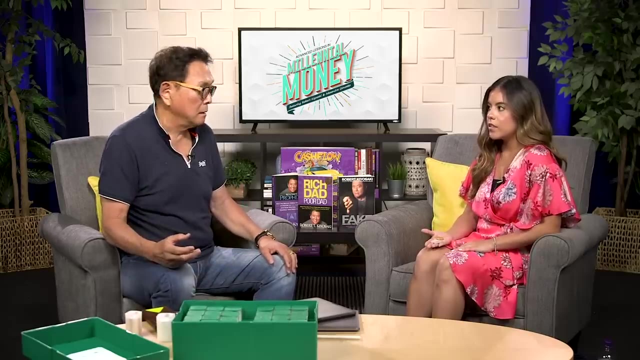 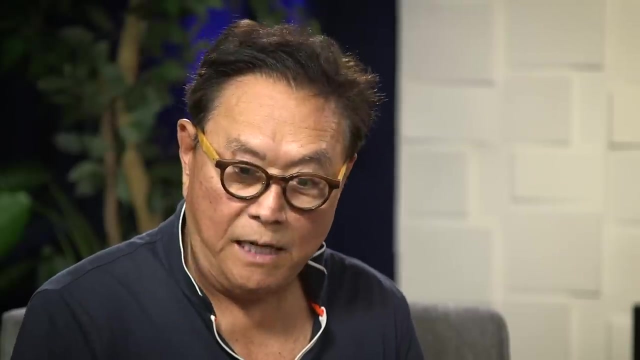 concerned, you're gonna find that most of my talks is about the Fed, so I would recommend you guys buy this stuff. don't buy it. don't save money. don't save government money, because they're corrupt as hell. as you know, save God's money in school. they compensate for a risk by telling you to. 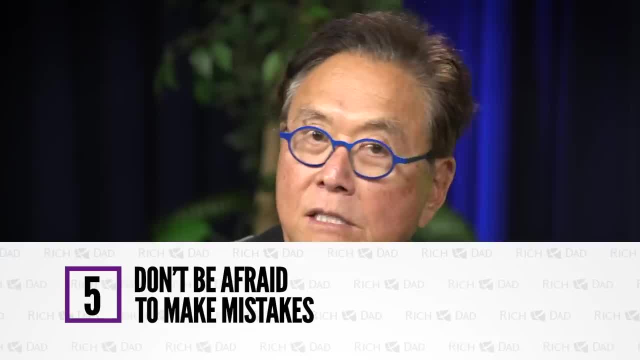 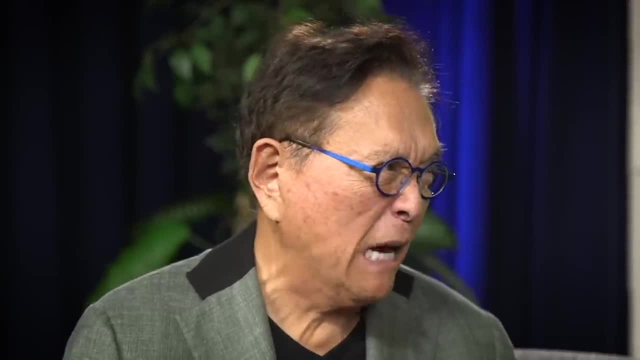 memorize the right answer. so, in other words, these kids leave the young people like you leave school, think, oh, if I know the right answers, then there's no risk. and it drives old guys like me crazy because everybody's talking about Millennials. what's wrong with them? 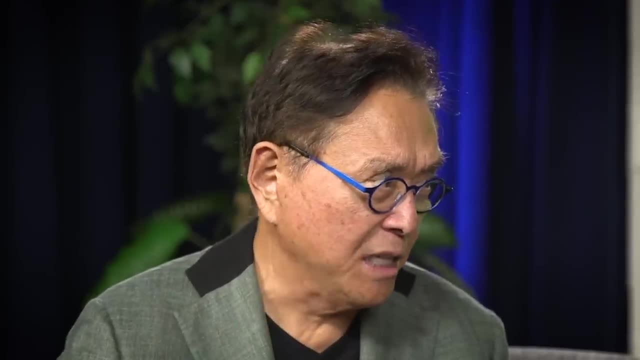 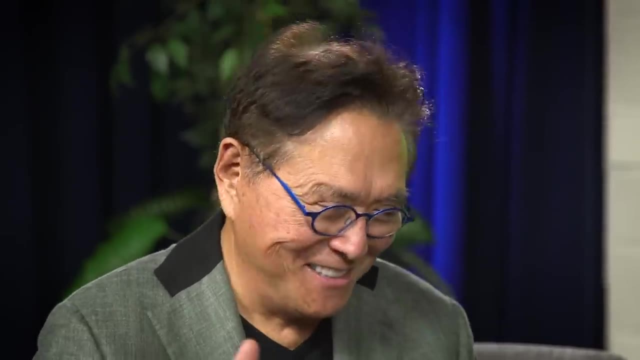 you know, Millennials are the most highly- in many ways the most highly- educated generation in history. they have the cell phone. they didn't get educated in school, they got educated on social media, on the cell phones. they know all the answers, but they're afraid of doing anything. yeah, you know the biggest. 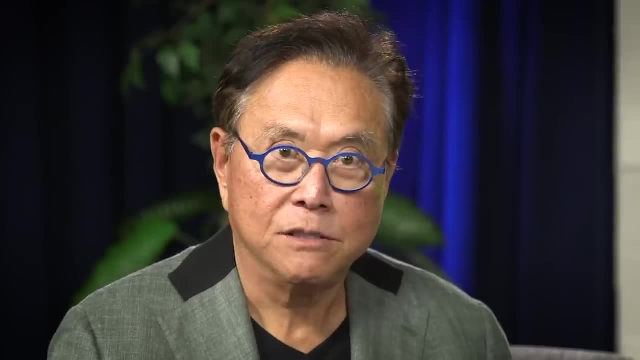 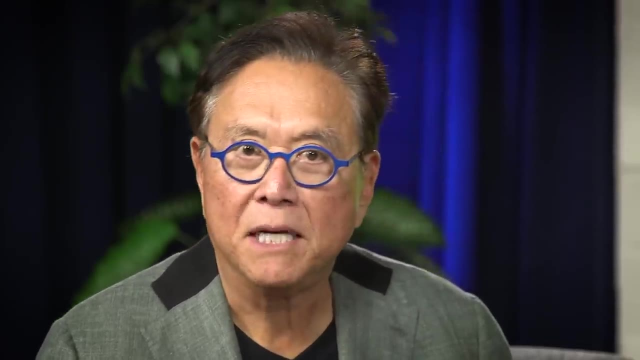 complaint about my generation is: Millennials know all the answers, but they can't do anything. the reason they can't do anything is because you might hurt there's somebody's feelings, you might make a mistake. you know there's a lot of things that they can't do and that keeps you guys just trapped in this. 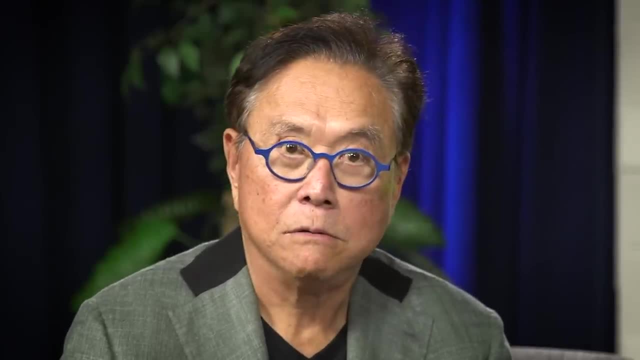 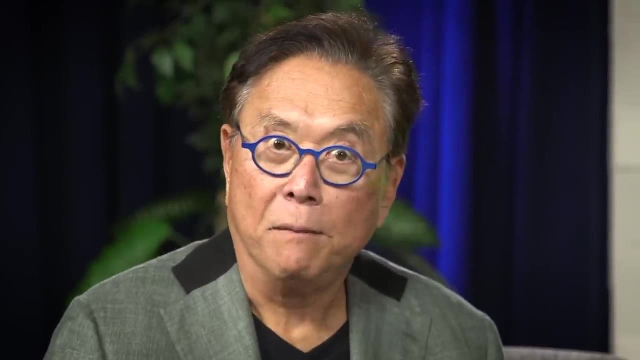 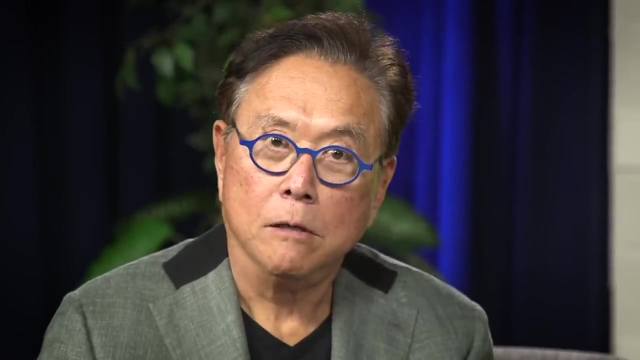 little box. yeah, so that's one of the reasons I think Millennial money is such an important point here, because if you're going to come into my world- old guys world or the information age- you've really got to understand what is risky and what is not risky. and in my world, if you play it safe, that makes you stupid. 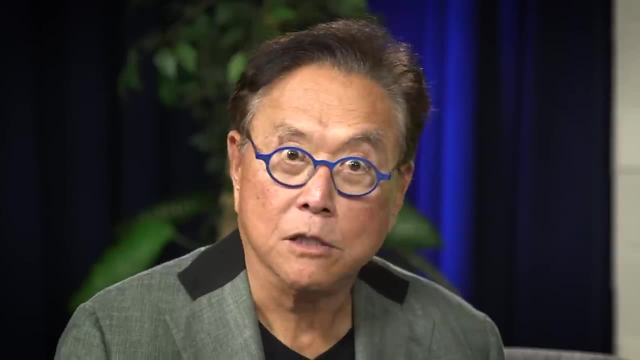 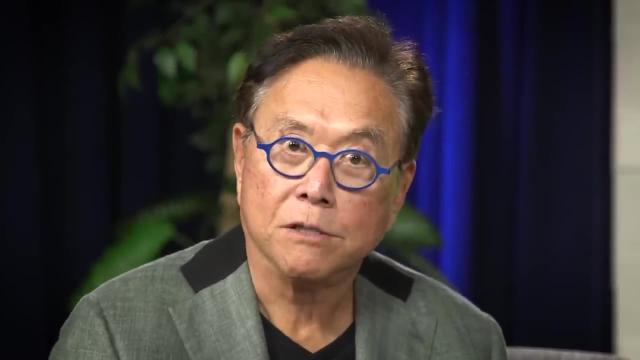 because if you don't take risks, you don't get smarter. yeah, you know, so you answer, but you can't do anything. yeah, and one of the best things I had is I went from, I went to military school, then I went to flight school. I had such great. 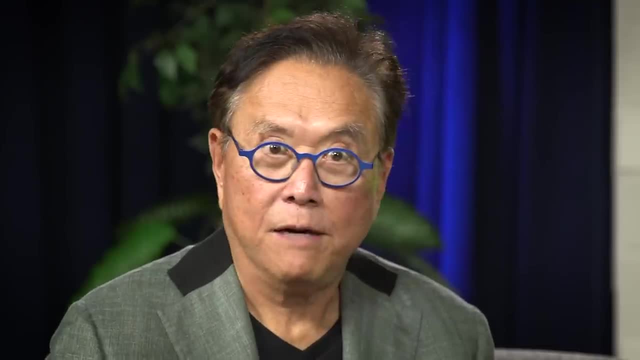 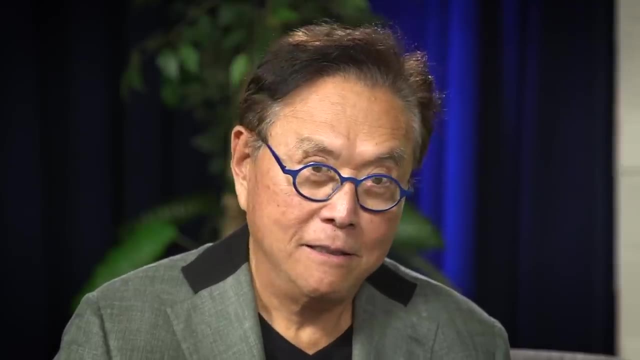 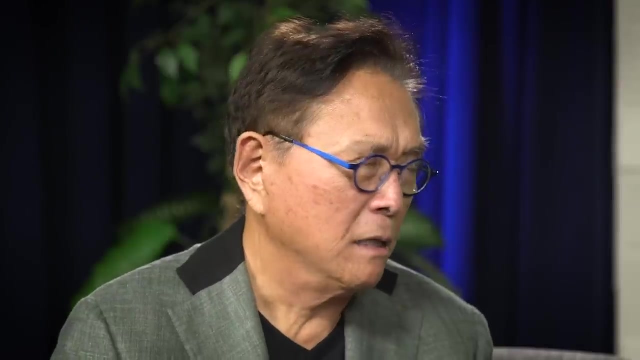 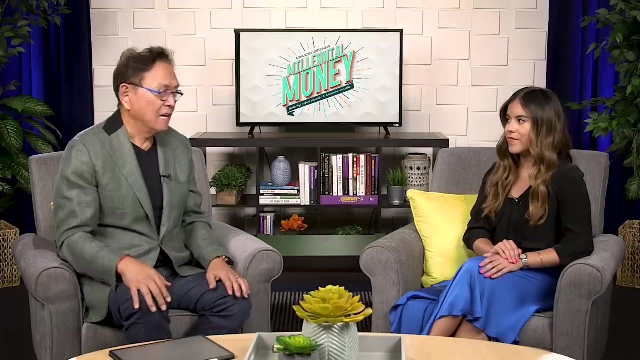 teachers. you know all of them could fly. you know so my flight instructor could fly. what a novel idea. you know a flight instructor can fly, but when I was in high school, most of my teachers were terrified. they're all cowards. you know job security, make mistakes. just memorize the right answer and you'll be safe. and that's why. 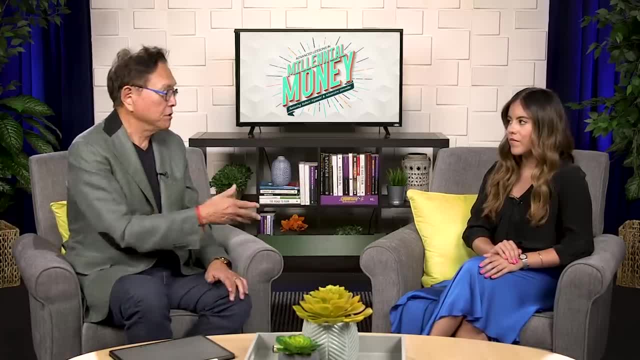 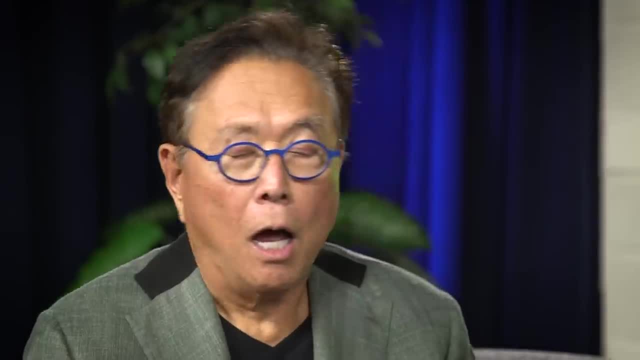 most school teachers aren't rich. yeah, they teach that to your generation, yeah, and most of them are teaching us things that they don't do on a daily basis, like we have entrepreneurship classes, oh, and they're not entrepreneurs, you know. so it's it's kind of frightening when you think we're relying on the school system. 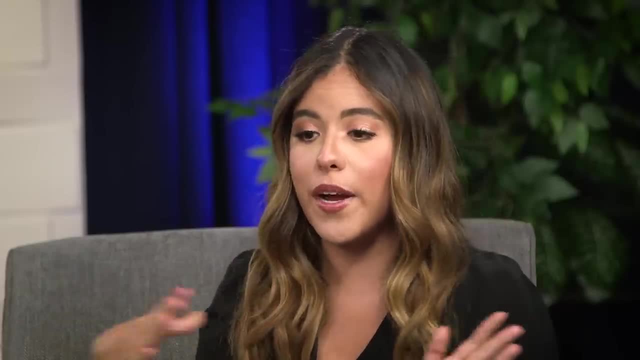 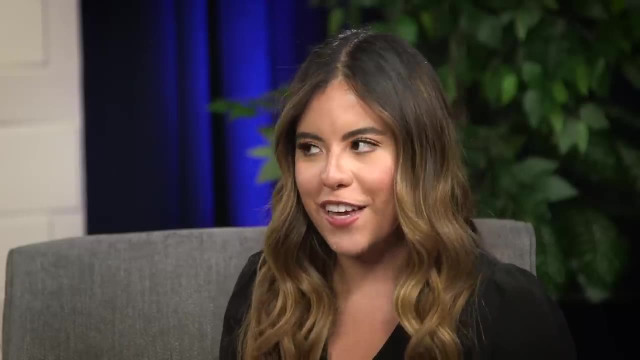 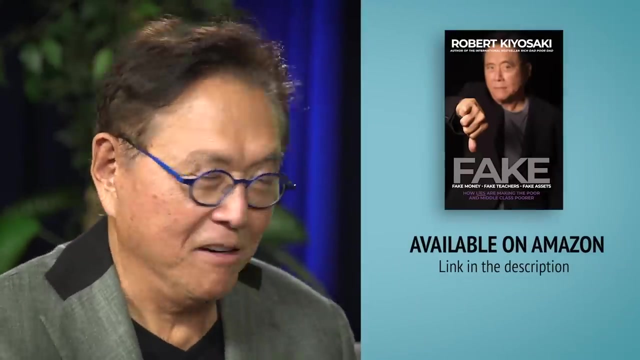 oh, and the fact that they're teaching us so the way to get through college right is practicing all the right answers, taking the exam, putting in all the right answers, when in real life that's the last thing that will ever happen, right? no, like you talk about fake, you know this is my book. fake here. fake money. 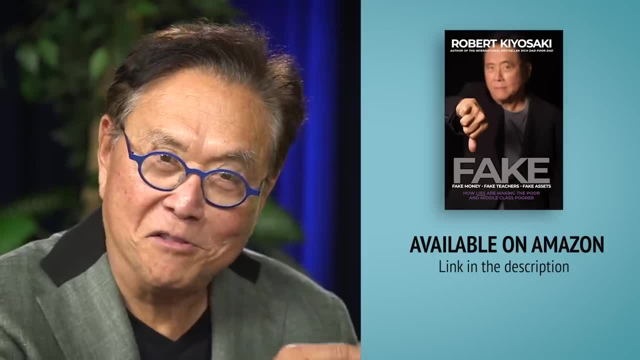 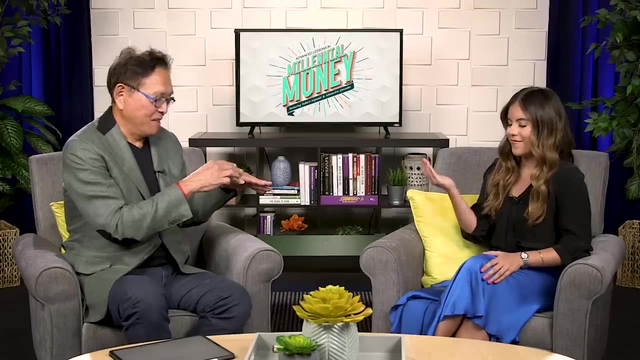 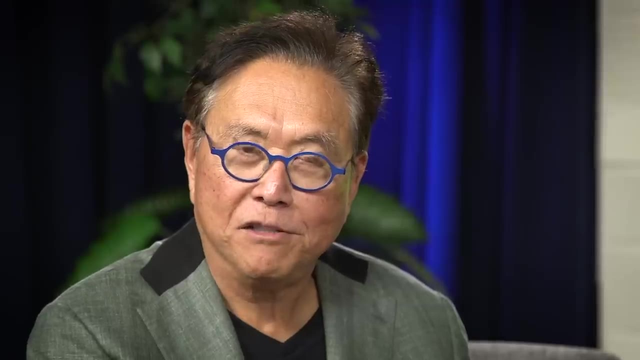 fake teachers, fake assets. the reason it's fake money, fake teachers and fake assets, it's because it all has to be fake. you have to have fake teachers to understand fake money. then you have to have fake assets to buy those stocks, bonds and mutual funds- fake assets, but without fake teachers. fake money: you. 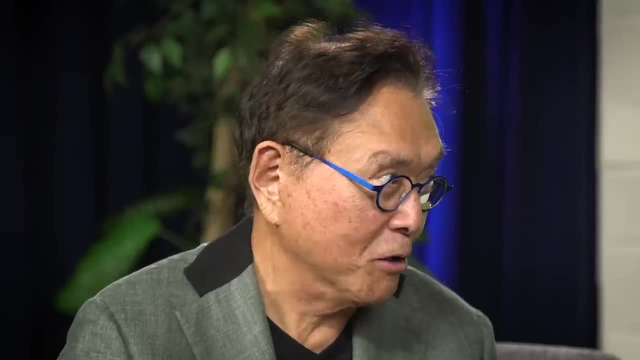 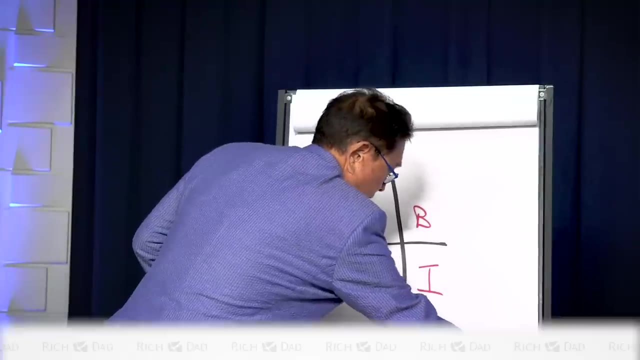 can't do it. so that's why I love, I love working with on these programs here, because if you're going to be successful, you've got to take some risk. most of the young people your age today, and a lot of them, want to become entrepreneurs. the problem with 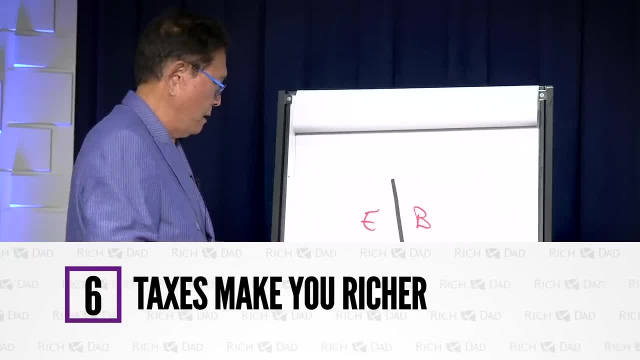 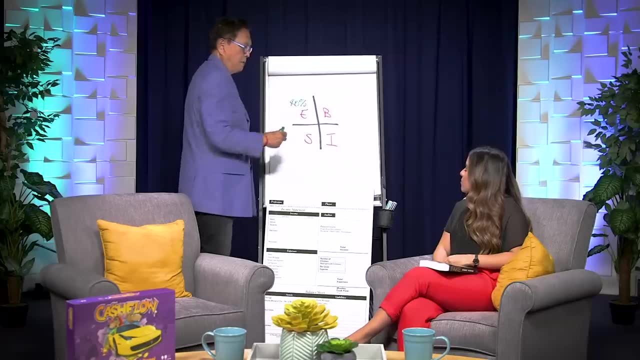 this. you have to understand tax. you see, this is all over the world, very little difference. these guys pay 40% of their money in taxes. so they make a thousand dollars, they're gonna spend four dollars in taxes. these guys that make a thousand, they're gonna pay 60% in tax. 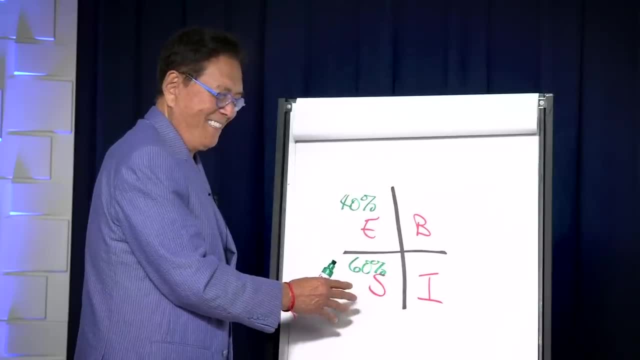 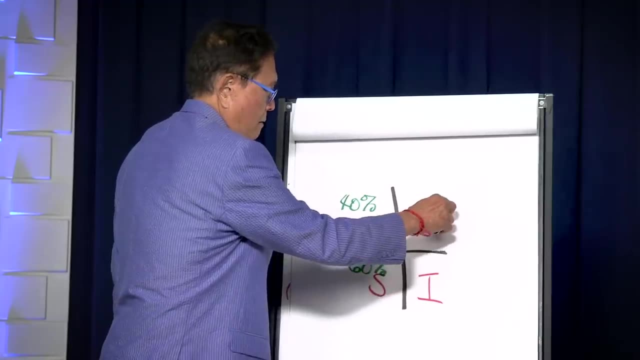 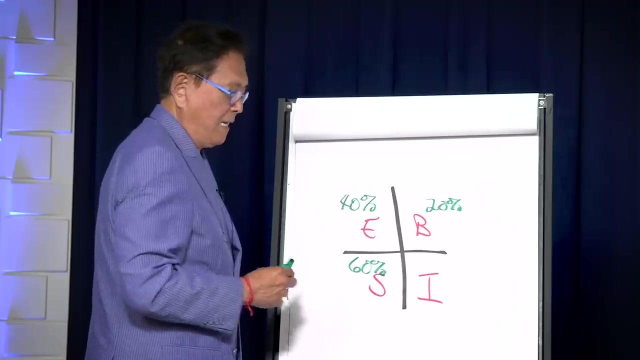 So our schools are teaching entrepreneurship, but they're not teaching them tax. okay, And because they're focusing on income Over here it's 20% in tax, So they make $1,000, only $200 goes to tax. 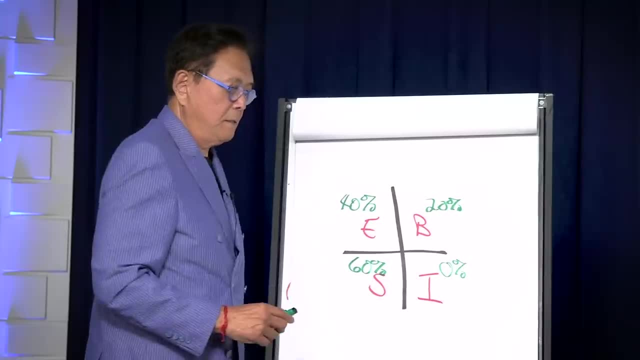 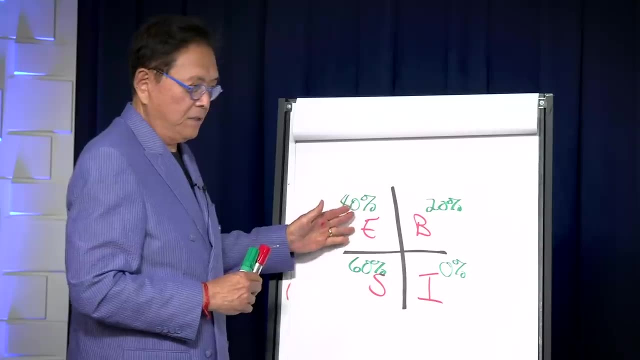 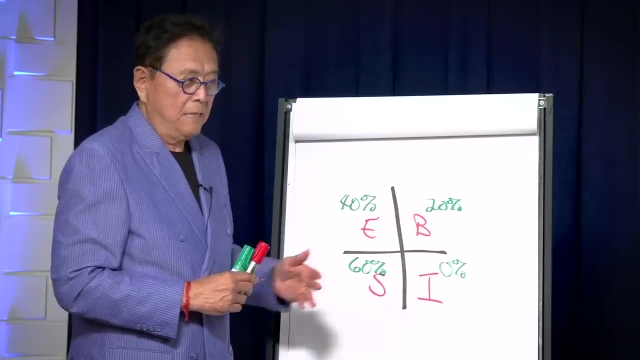 And these guys 0%. So the reason financial education isn't working in our school systems is they're teaching financial education for these people and these people. but to really become rich, you have to focus on this side here, And that's the difference between a rich dad. 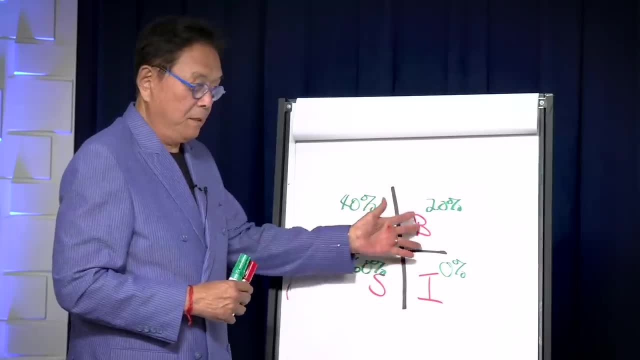 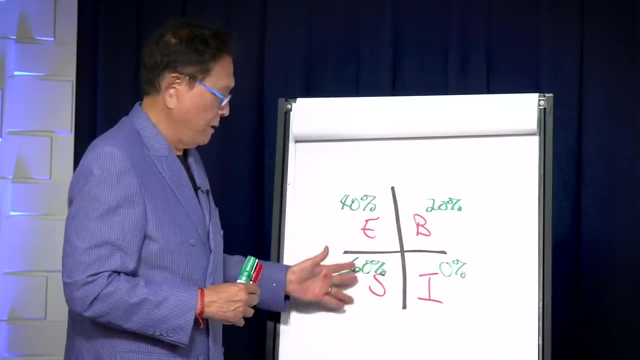 and what they're teaching in school. right now I'd rather be on this side. This side is a lot harder, but in the long run it's more fun for me On this side. here it's harder, but you're paying tax constantly. 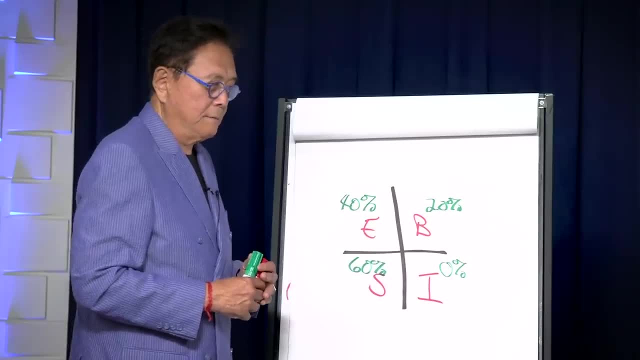 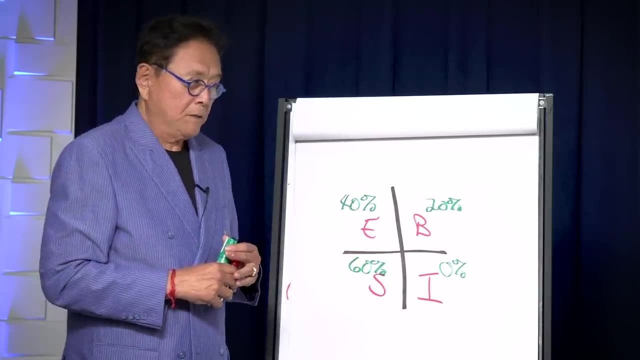 So these guys here are saying: when taxed or rich, well, these guys don't pay taxes. And as strange as that may seem- and I'm talking about legal this is all over the world, So that's the big difference here. 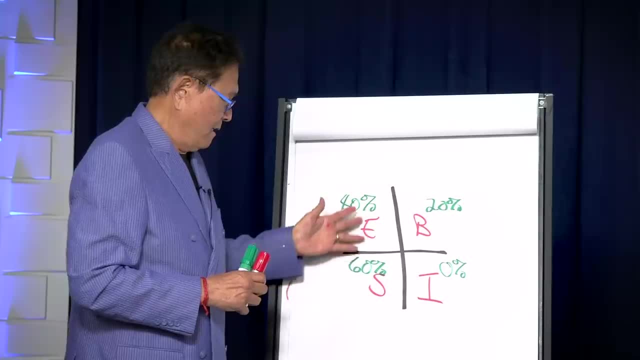 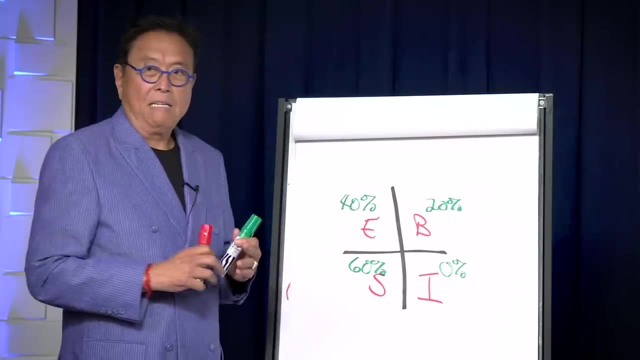 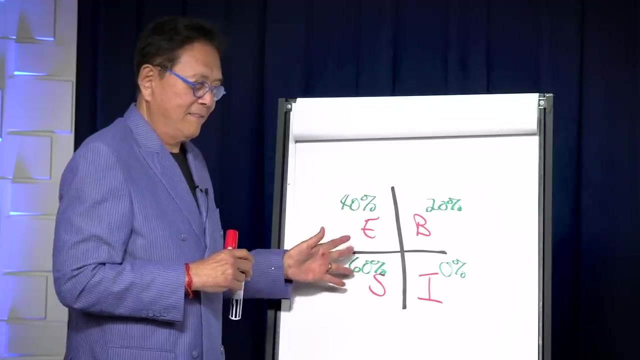 One last thing which I think most millennials understand is in Rich Dad, Poor Dad. I wrote about Ray Kroc, founder of McDonald's, And he was teaching at the University of Texas the MBA program, and Ray asked and most of the MBAs are gonna come out here. 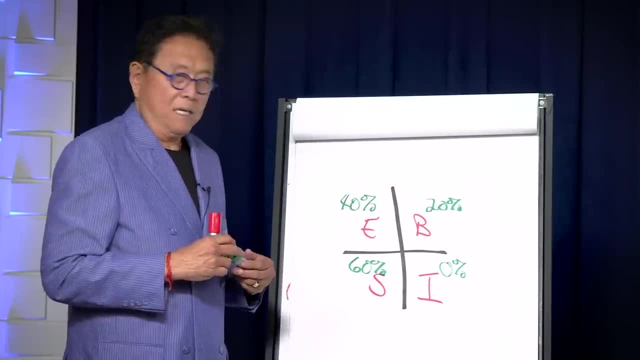 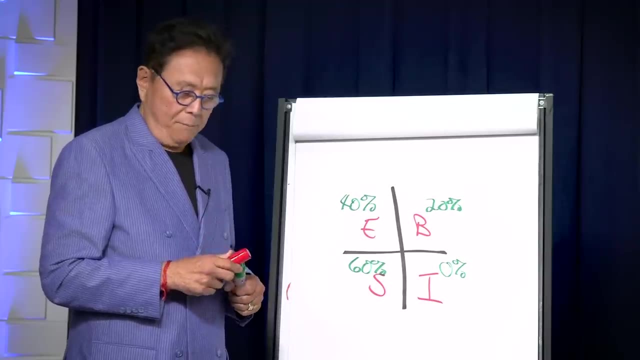 Ray Kroc asked him. he says what business is McDonald's in? And everybody yelled and said no, no, no, we know you're in hamburgers. And Ray says no, McDonald's is not hamburgers, McDonald's is in the business of real estate over here. 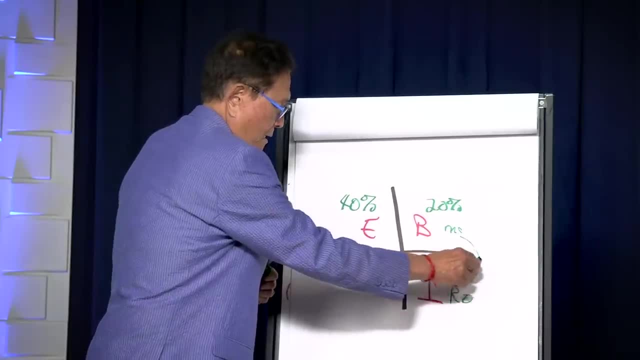 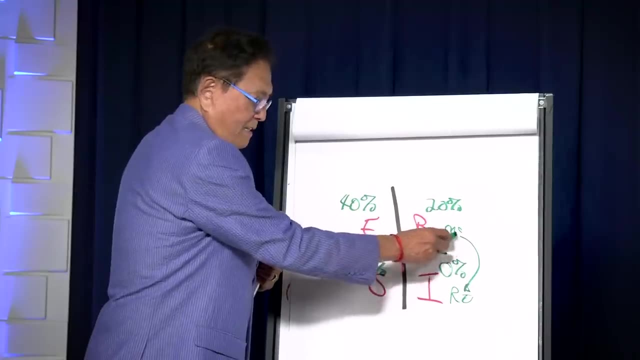 So you have McDonald's here and the money McDonald's makes buys the real estate. And that is my formula. This is Rich Dad, I own real estate. I don't hang out here. I'm glad you guys are here, right. 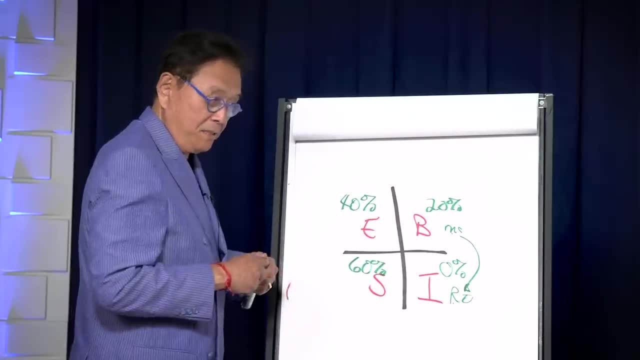 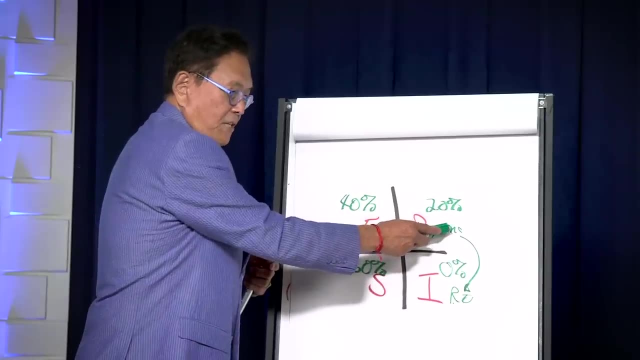 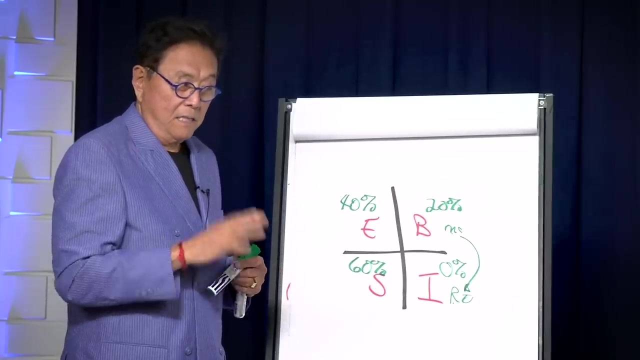 And we do our best to make sure you're educated and you have your own businesses and things like this here. But really the formula I follow personally is McDonald's- We have education company that buys real estate, which means we make a lot of money, pay zero taxes legally. 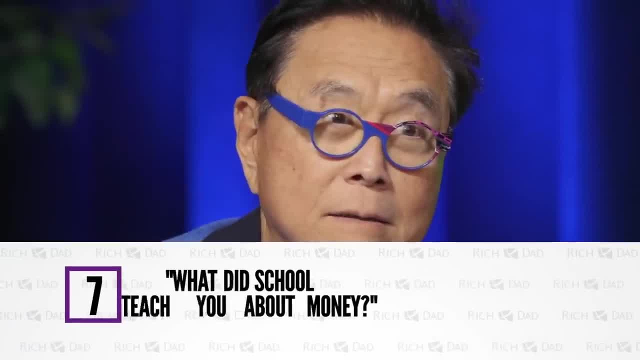 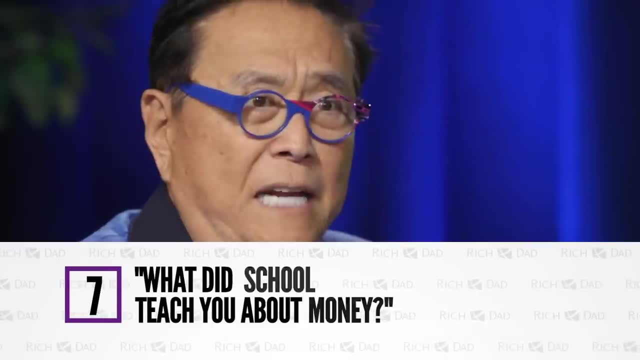 What does school teach you about money? Nothing, I mean. give me a break. Give me a break. So the other part of when you look at this financial statement up here, that's what your banker wants to see. Your banker doesn't care about your grades. 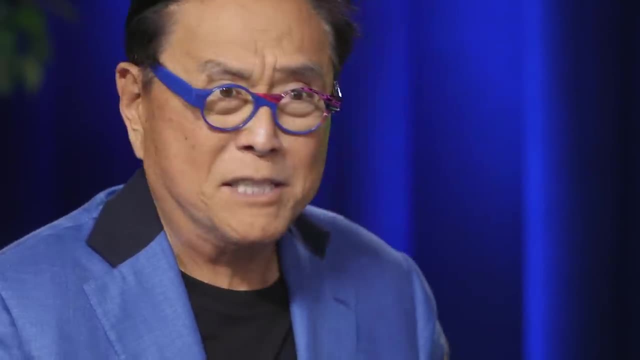 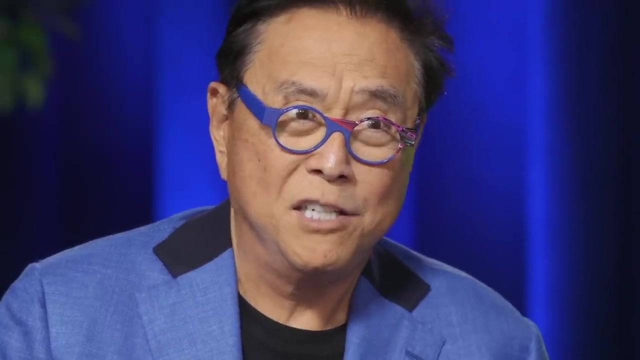 Banker doesn't care what school you went to. I meet so many people say, oh, my banker won't give me any money, Says well, cause you don't have one of these. And when you look at most of the politicians today, they don't have one of these either. The US government doesn't have one of these anymore. They stopped doing this Cause of the US government. the budget is so out of balance they can't do anything. So that's why, you know, 22 years ago, in 1996,. 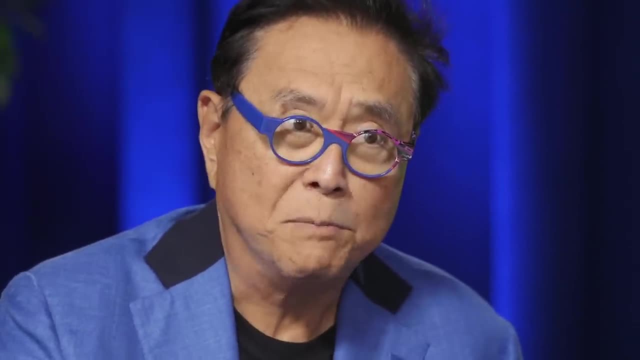 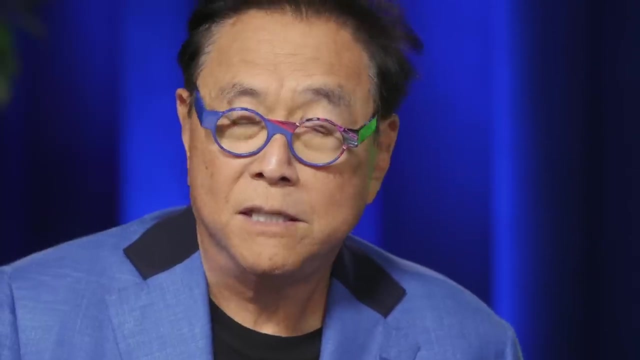 I created the cashflow board game. The purpose of this? so people could teach people what our school systems will never teach you. Never. because they don't know it, Because evidence is now coming out that the school system was hijacked by the ultra rich. 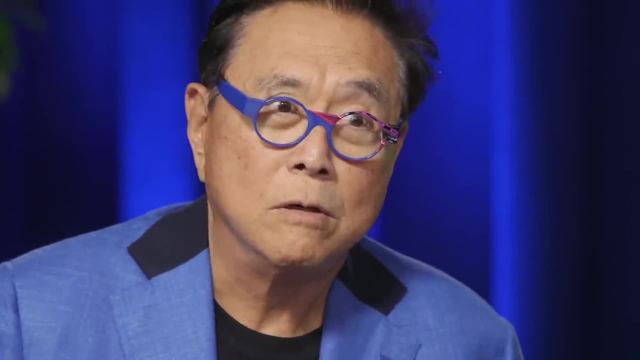 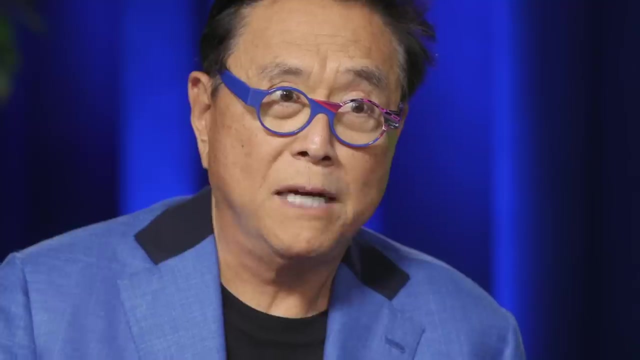 years and years ago to never teach people what I know, What my rich dad taught me. So that's why most of our political leaders are broke. They're poor people. You know who makes the most of the politicians: They got paychecks for life. 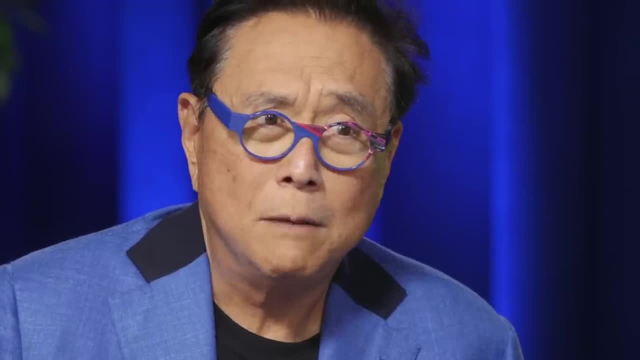 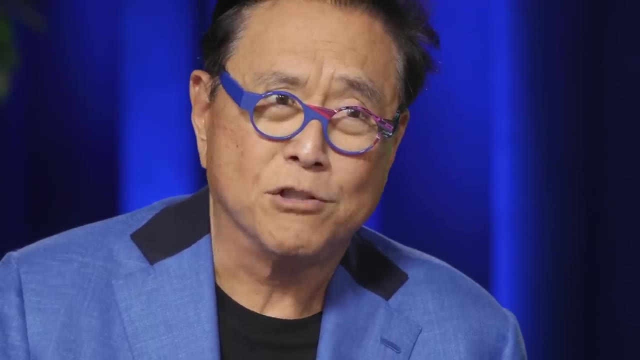 They get benefits for life and they got all this stuff, but they're doing a horrible job, So you're going to depend upon the government to take care of you. That's crazy. You know a lot of people don't like Trump.